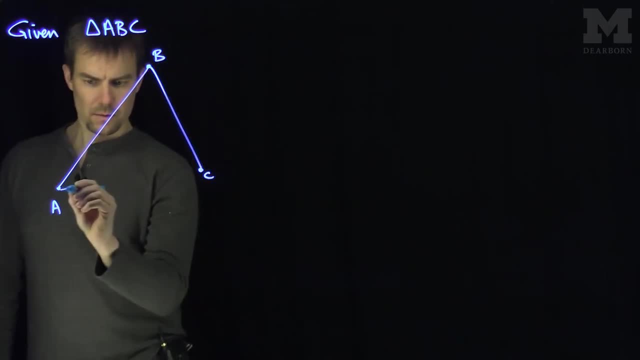 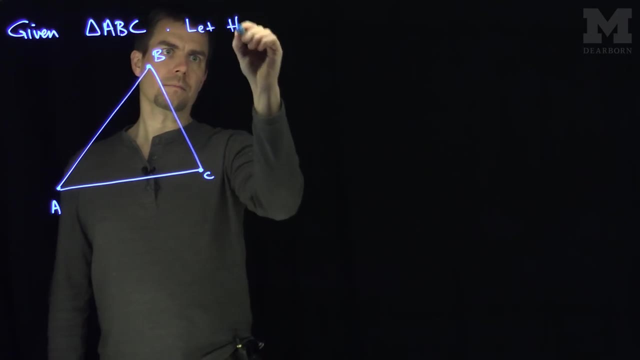 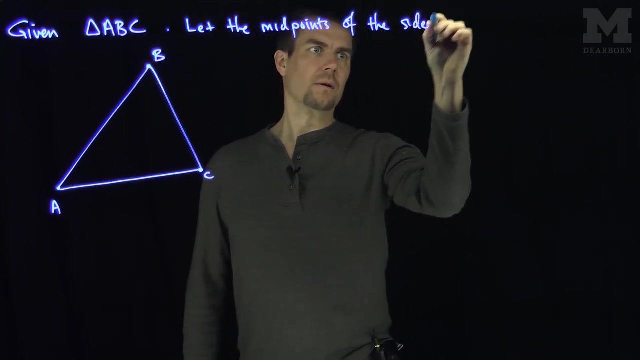 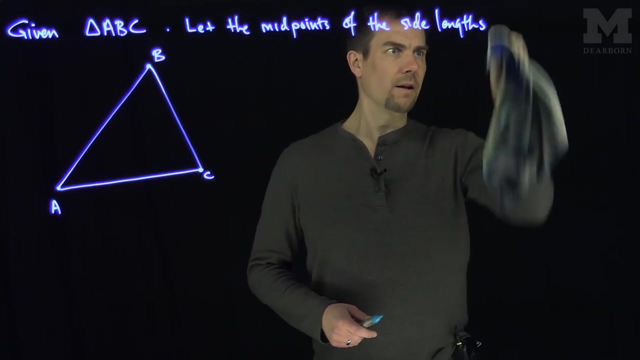 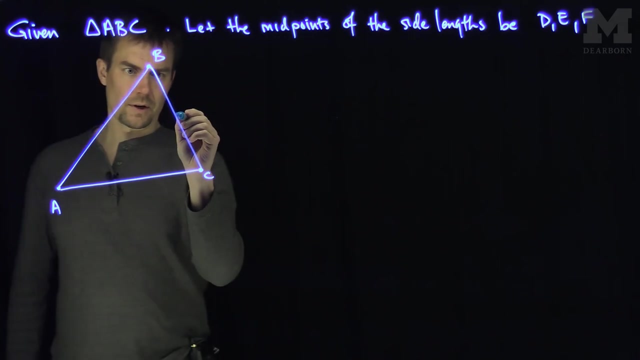 down to a point over here, C. Let's plot the midpoints of the side lengths B, B, D, E and F. So let's let them be D, E and F. Okay, So what I'll do is I'm going to call this point over here, opposite from A. I'm going 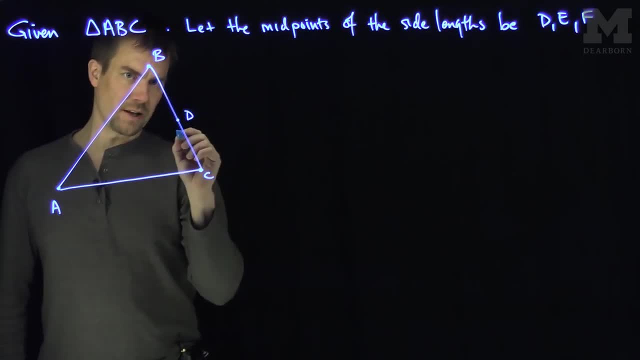 to draw this as best I can. That's like the midpoint over here. Let's call it midpoint D, And over here are the midpoint of A and C. So that's going to be. we'll call that point over here E. That's another midpoint. Of course, we know that this length is this. 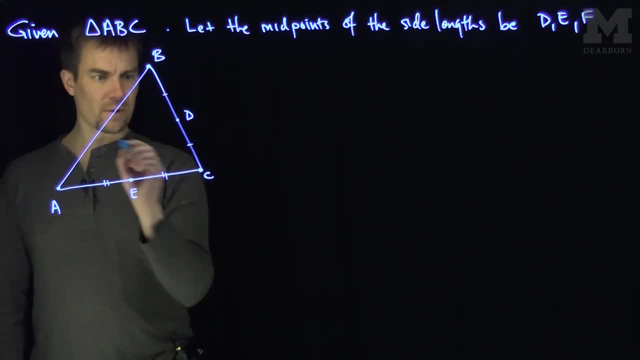 length, so it is a midpoint, and that this length over here is this length, so it's a midpoint. And finally, we have the point F over here. that's more than the midpoint right about there. That's the point F and we know that this length is this length right. 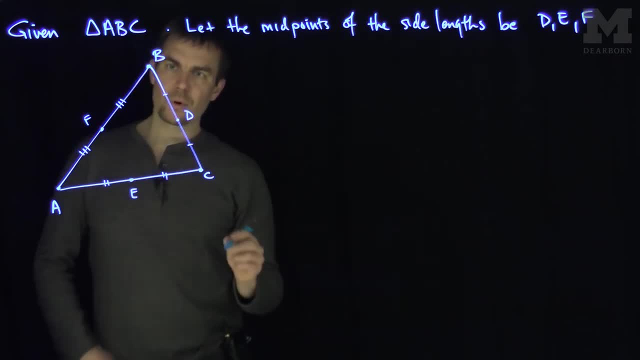 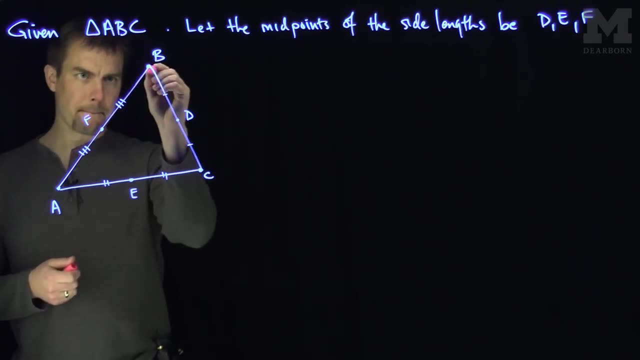 over here. So we have the three midpoints right, And so what I'm going to do is I'm going to consider the intersection. so I'm gonna draw this first savion from B to E, and then I'm gonna draw the line from A. 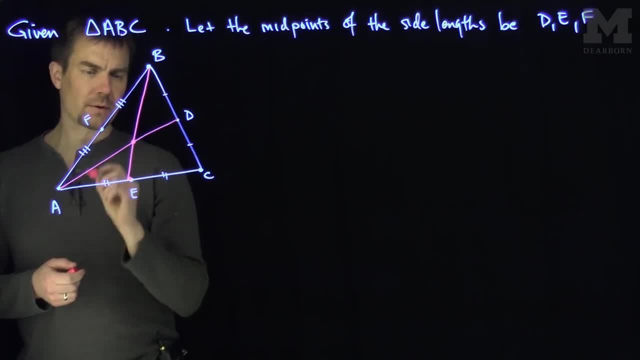 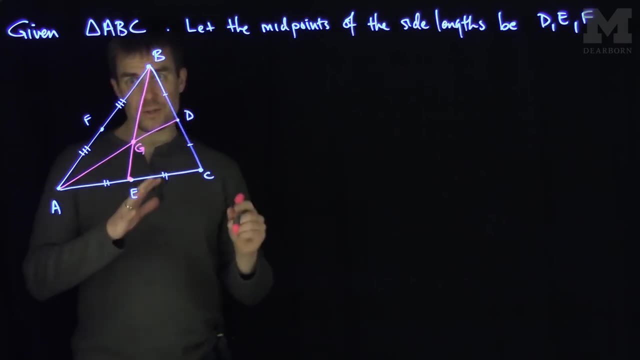 the savion from A to D right, And they're gonna intersect. those two lines are gonna intersect at a point which I'm gonna call G over here. And so now what we're gonna do is the following: We're going to find a representation of the vector point G. 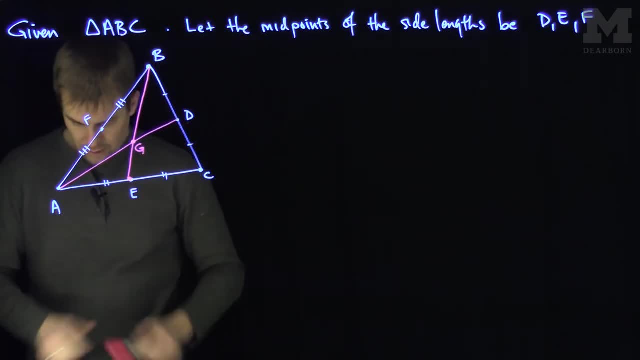 Now we can think of each of these points, each of these vertices of the triangle as a vector right. We can think of the origin as over here. So say, for example, here's the origin and then this point over here A. 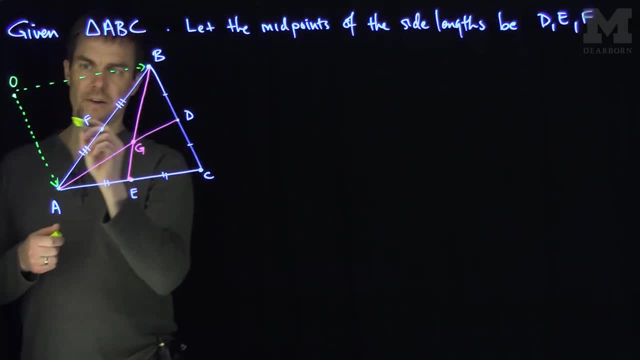 is really genuinely in a vector. That point B is genuinely a vector. The point C- I don't wanna mess up the figure too much, but I could draw from the origin to C- and that's a vector over here- And I can also draw from the origin to G. 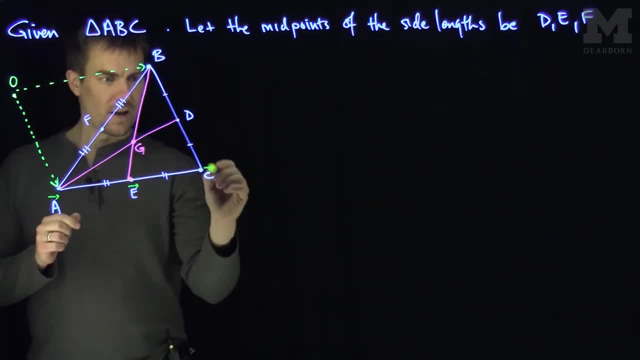 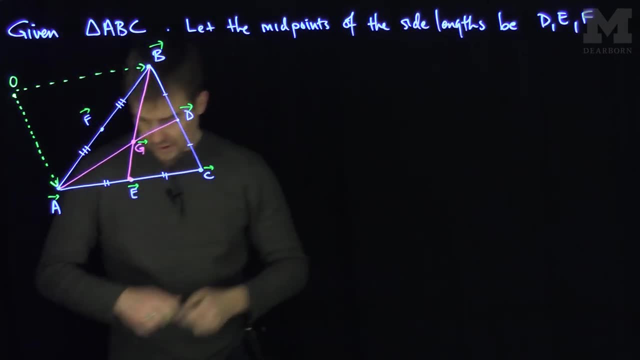 And so all of these things are really vectors, right? So these are vector points over here, And we have representation of these vector points too, right? And we have the vector representations of all of these things. So, for example, we know what the vector E is. 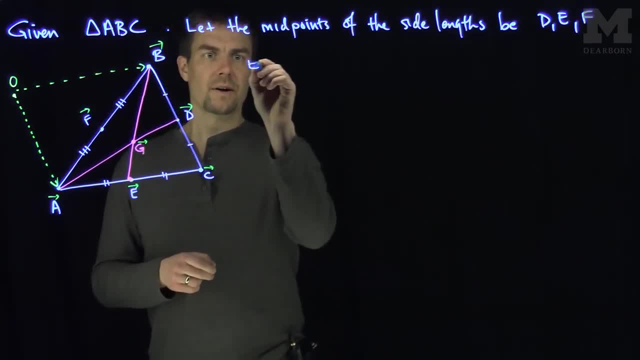 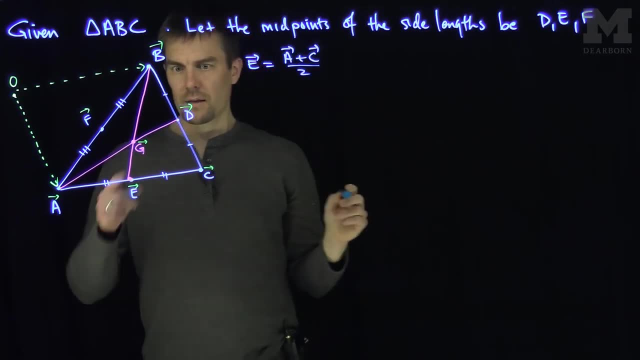 We know that the vector E, for example, is the midpoint of A and C. so the vector E is really the vector A plus the vector C over two. That's the midpoint formula. The vector D is going to be, is gonna be, the midpoint of B and C. 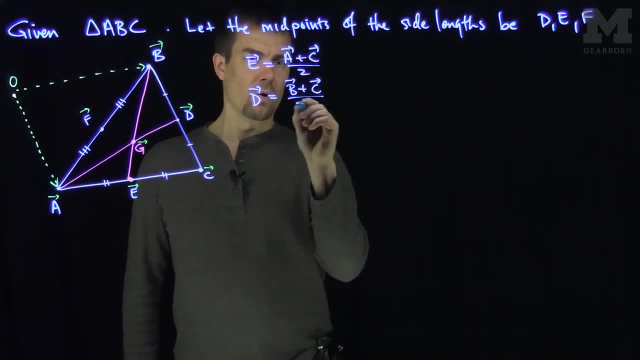 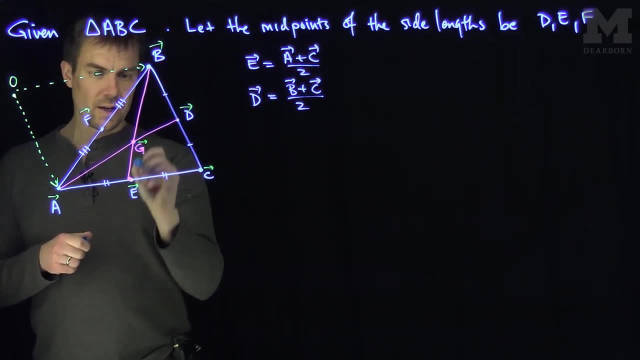 so that's gonna be B plus C over two. And so now what we know from this configuration is: we know that the vector from B to G is in the same direction as the vector from B to E. So if I look at this vector over here, 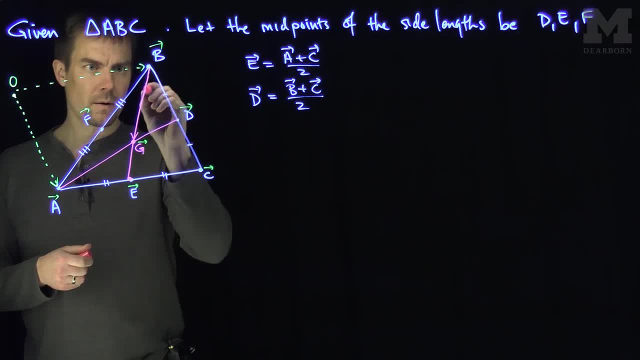 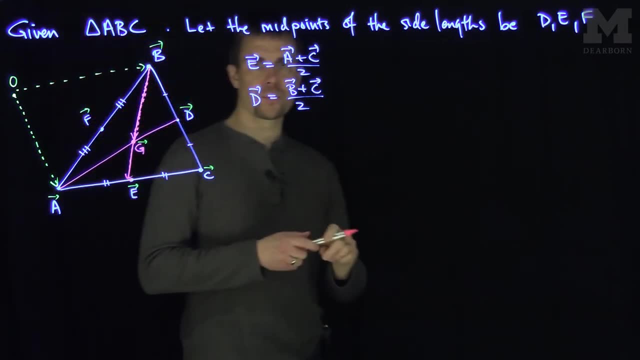 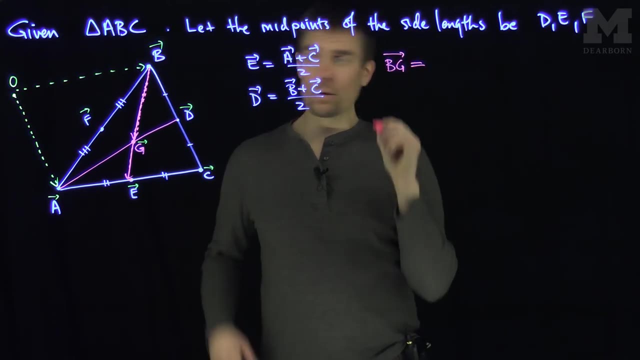 so this vector from B to G is in the same direction as the vector from B to E. So, in other words, what we have over here is we have that the vector BG is a multiple of the vector B to E. So I'm gonna call that first multiple over here lambda one. 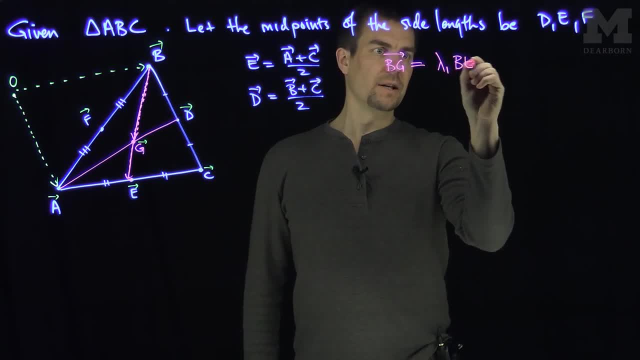 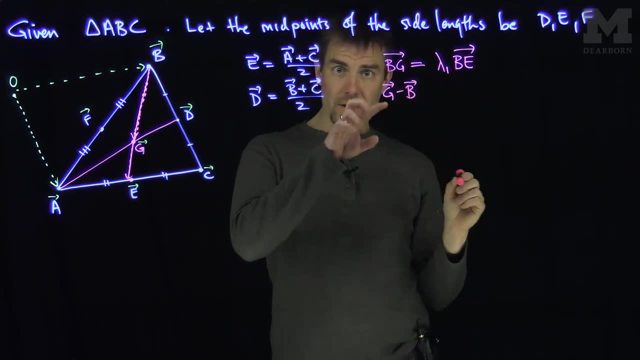 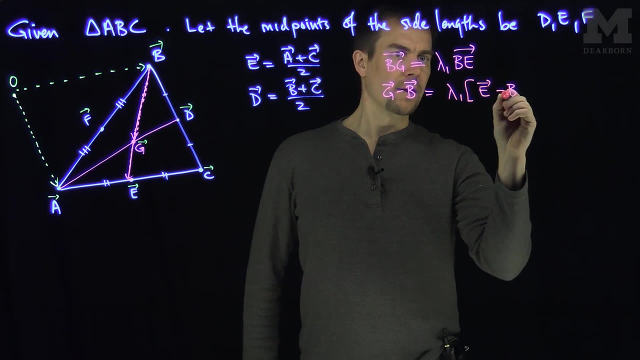 So it's a multiple, a scalar multiple, of the vector B to E. right, So now what is BG? That is, the vector G minus the vector B. It's the endpoint. It's the endpoint minus the initial point for vectors. And then lambda, the vector E minus the vector B. 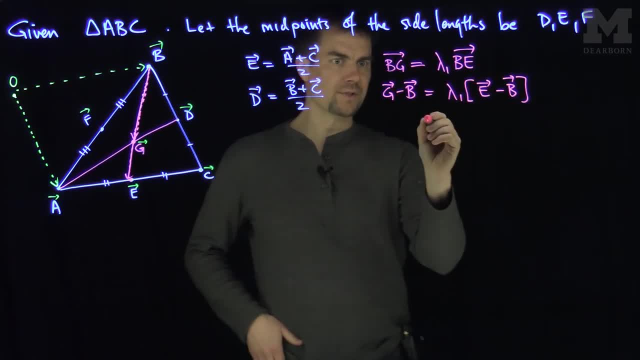 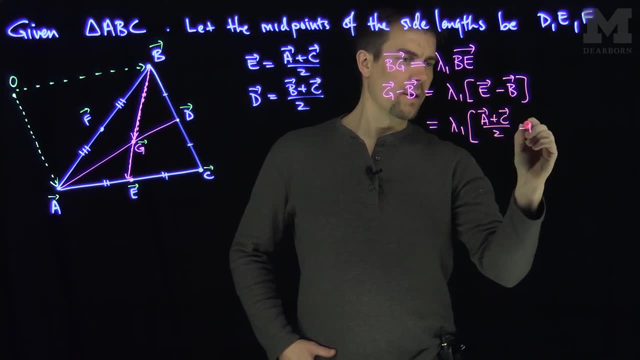 Now we know what E is. E is gonna be A plus C over two. so let's simplify this. This is going to be lambda one, and then I'm gonna have an A plus C over two, minus B, And so if we do one last simplification- 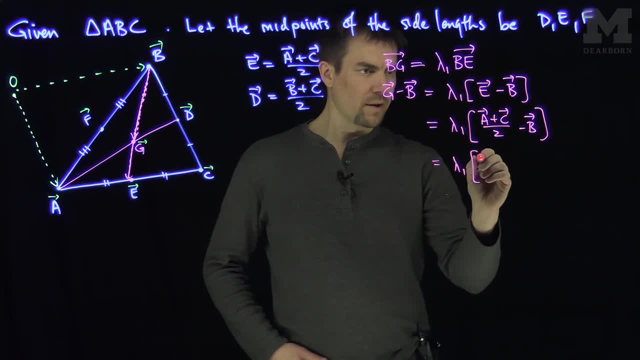 we have lambda one, and then we're gonna have a lambda one, and then we're gonna have an A plus C over two minus B. So I'm gonna have an A over two. That's my A component. I'm gonna have a lambda one, C over two. 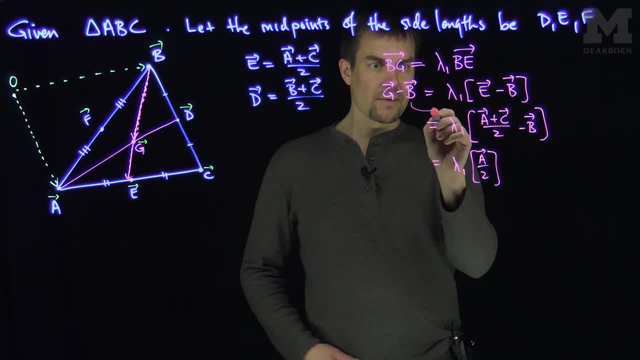 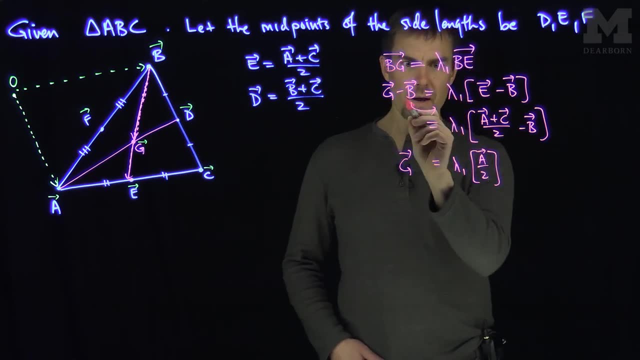 and I'll see what happens over here. We're gonna have a. I can throw this B on the other side of the equation and then I'll have what. Then I'm going to have a one minus lambda one B. So I'm gonna have a plus one minus lambda one. 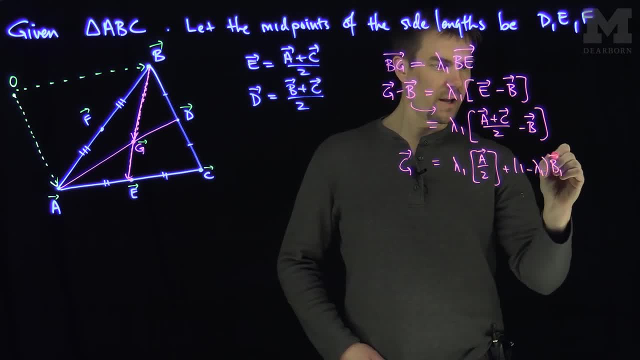 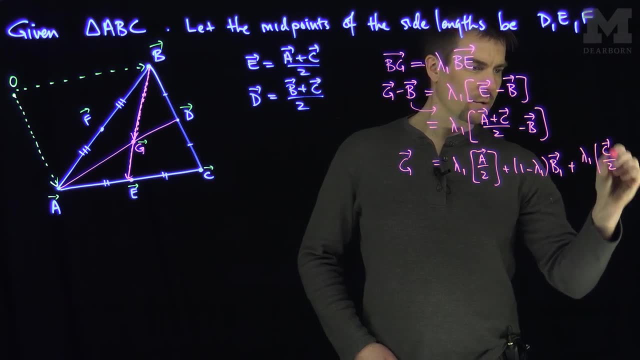 one from this B over here, and then a negative lambda one in the direction of B, And then we'll have a. what We'll have? a lambda one, C over two, plus lambda one, and then that times C over two. So this is one representation of my vector G for the median. 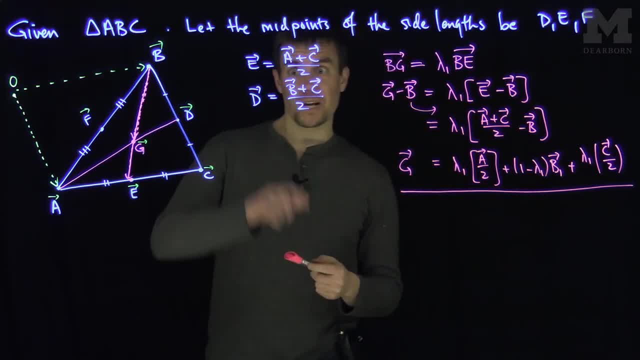 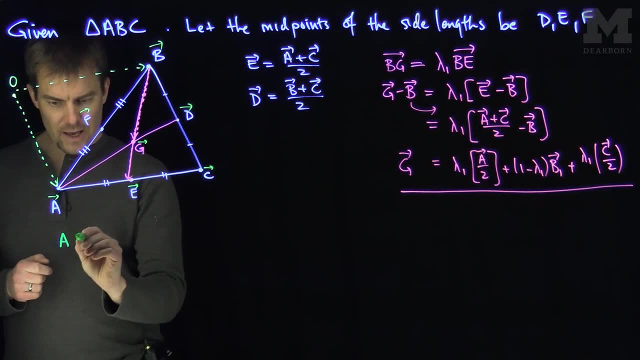 It's this representation over here. I can also write down a second representation in terms of this: A to D, right. So we also know similarly that from A to G. I know that A G, that vector A to G, is in the same direction. 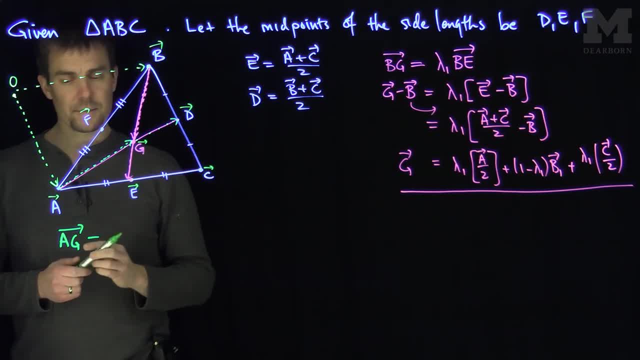 as A to D. So this is gonna be another multiple, maybe perhaps a different multiple. We don't know a priori that it's the same multiple. yet. Lambda two, and then what? And then the vector A to D. Okay, 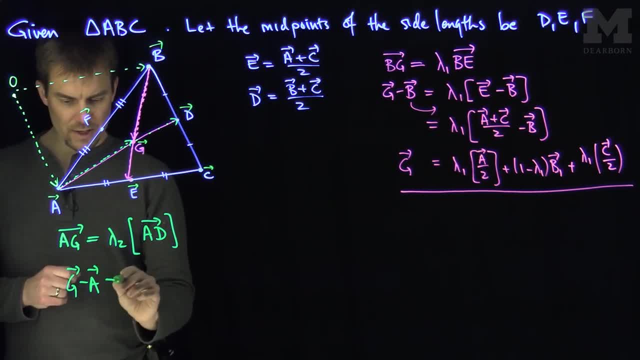 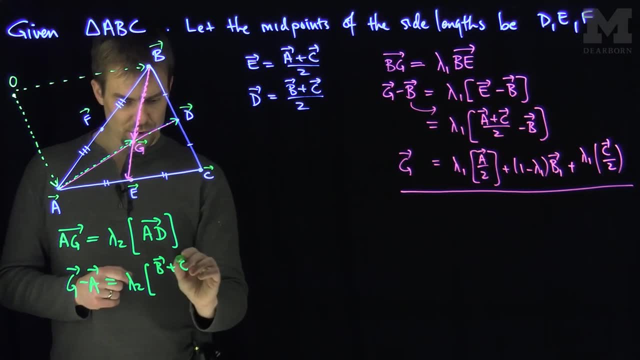 So this is gonna be G minus A. over here on the left-hand side of the equation is lambda two. And then we're gonna have D, which is B plus C over two. So that's gonna be a B plus C over two. 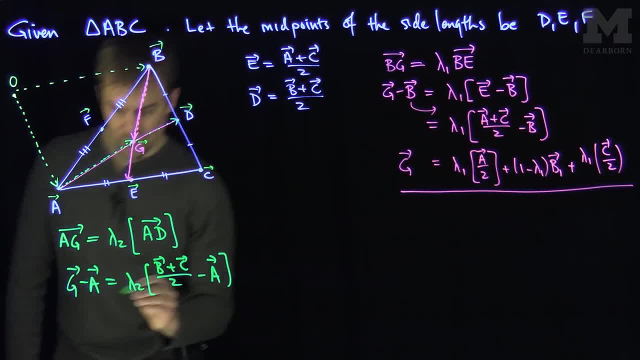 and then minus A. So by the exact same calculation, we can conclude from this that G is equal to. let's count. So I'm gonna have a one minus lambda, one minus lambda, two times the vector A, and then I'm going to have a lambda two. 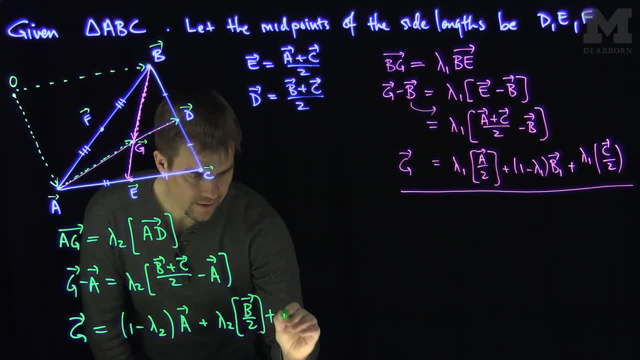 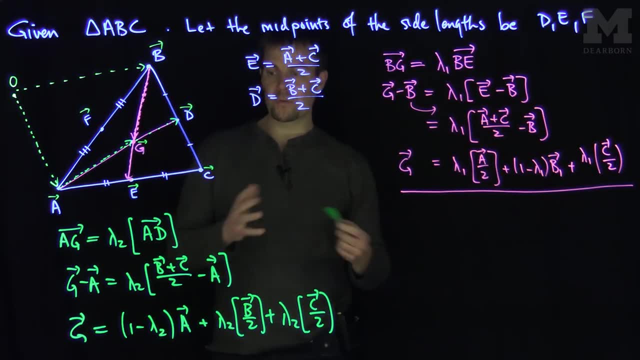 times the vector B over two. and then lambda, two times the vector C over two. So the conclusion from this is I have two different representations of G. Now the vectors A, B and C are in a triangle, so each of those vectors are going to be dependent. 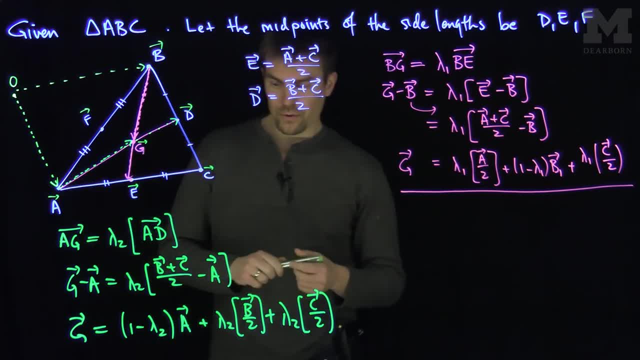 so they actually form a triangle, So they're independent of each other. So my conclusion from this is that all of these coefficients have to match up. So the conclusion from this, if we look carefully. let's look over here. So look at the coefficient of C. 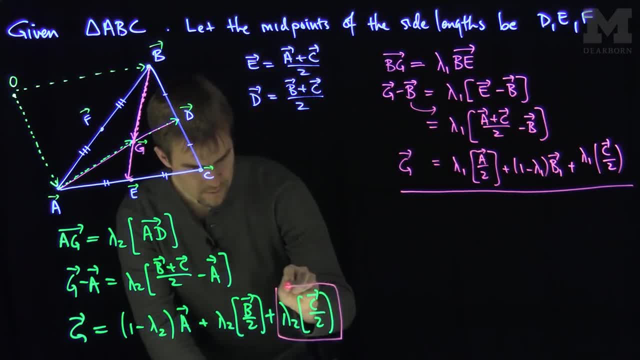 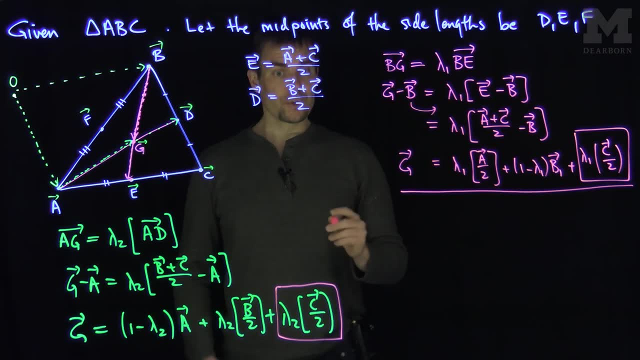 The coefficient of C is lambda- two over two, and the coefficient of C over here is what Is lambda, one over two? So those coefficients have to be equal. They're both the coefficient of C in an independent collection, of vector collection, And so our conclusion from this is: 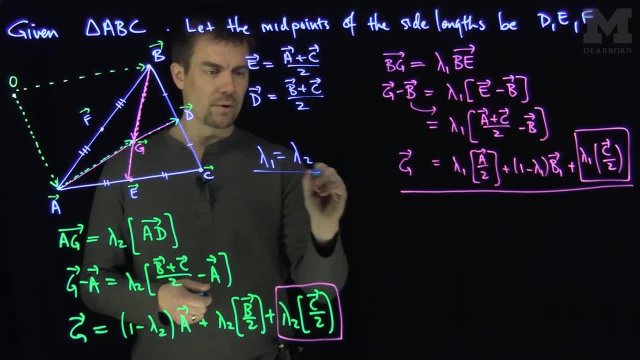 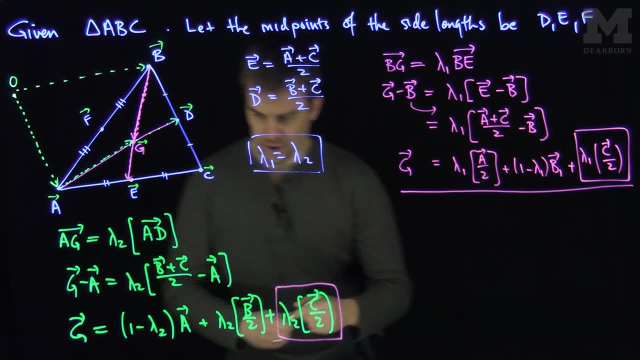 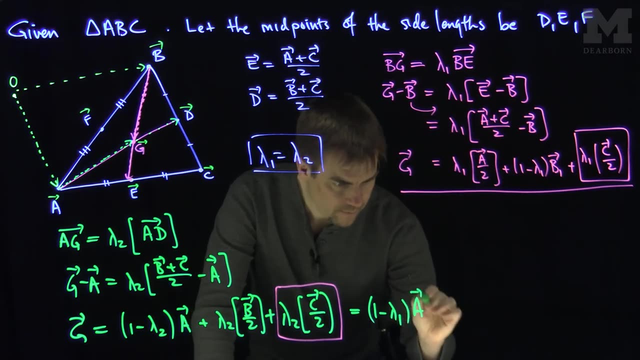 that lambda one is equal to lambda two. So lambda one is equal to lambda two. So this second representation over here we can rewrite it in the following way: The second representation is really what Is really: one minus lambda one, A and then plus lambda one and then B over two. 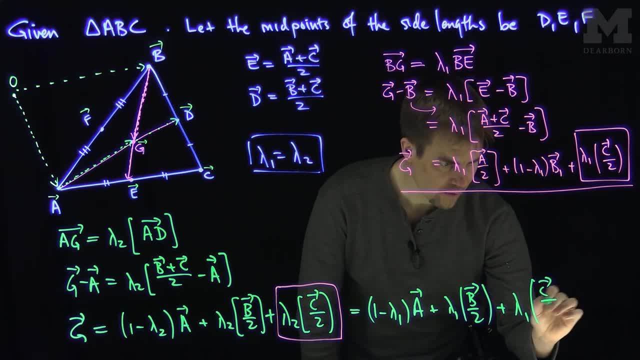 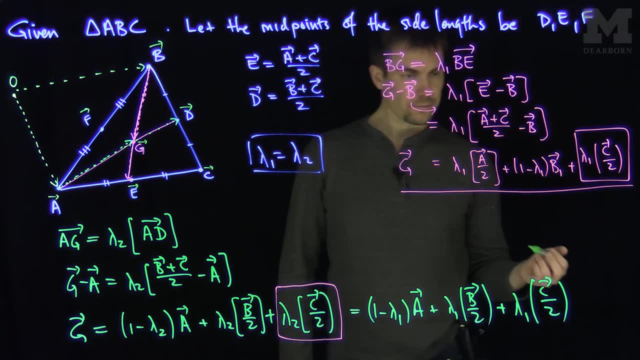 and then plus lambda, one C over two. So now I have two representations for G. They have to be the same representation. So look at this equation over here. So it must be the case that what It must be the case that these coefficients over here.